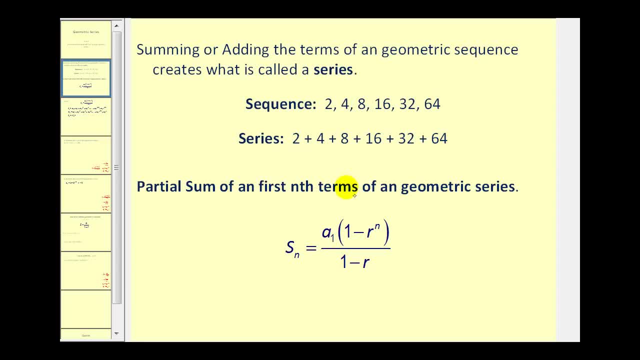 series is a sum. The partial sum of the first nth terms of a geometric series is given by this formula: S sub n is equal to a sub 1 times the quantity 1 minus r, to the power of n divided by 1 minus r. Let's go and take a look at where this 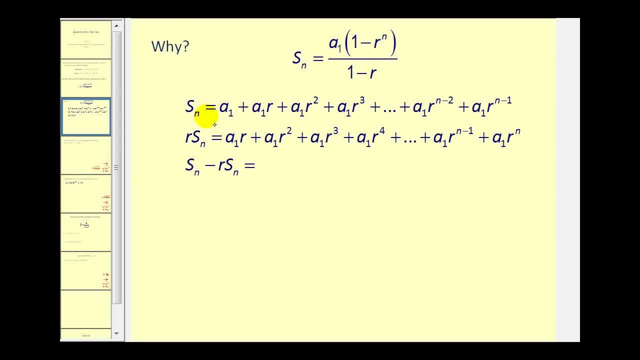 formula comes from If we were to start with the following geometric series, as we see here, a sub 1 plus a sub 1 times r plus a sub 1 times r squared, and so on, all the way out to a sub 1 times r, to the power of n minus 1.. If we take this, 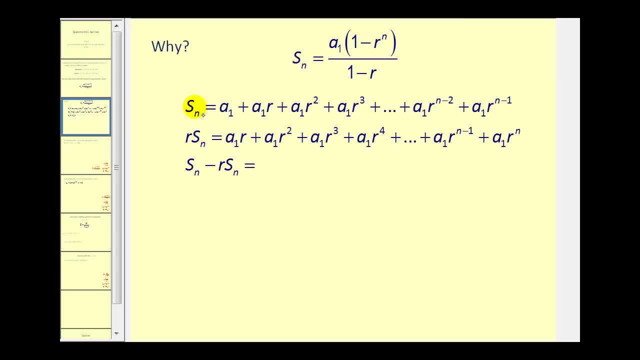 first equation and multiply it- both sides of the equation- by r, we would have: r times s is equal to, and each of these terms picks up an extra factor of r. So now the first term is a sub 1 times r, and the last term, instead of a sub 1 times r to the n minus 1, would be a sub 1. 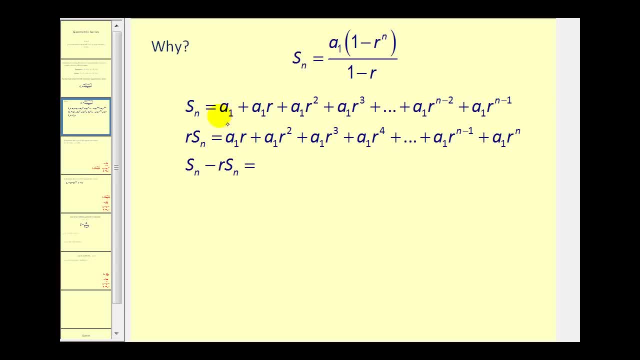 times r to the power of n. Next, what we're going to do is subtract these two equations. We're going to have s sub n minus r times s sub n, and if we do this, most of the terms will simplify out. for example, here we'd have a sub 1 times r minus a sub 1 times r, a sub 1. 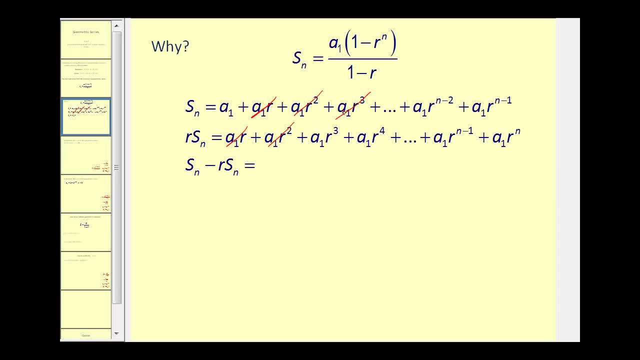 times r squared, minus a sub 1 r squared, and so on all the way out to the end, where we'd be left with a sub 1 times r to the power of n. So this difference will be equal to a sub 1 minus a sub 1 r to the power of n. Now, if we take the left, 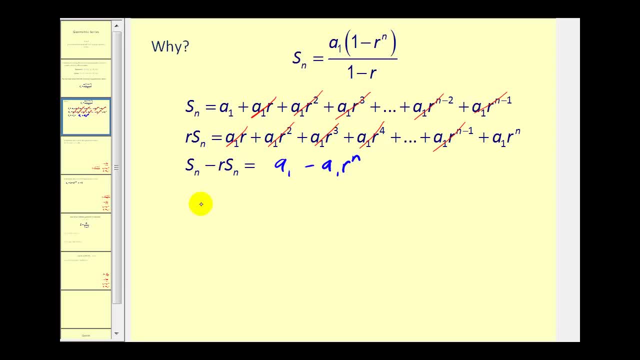 side of the equation and factor out the common factor of s sub n, we'd have s sub n times the quantity 1 minus r equals a sub 1 minus a sub 1 r to the power of n. Now we could divide both sides of the. 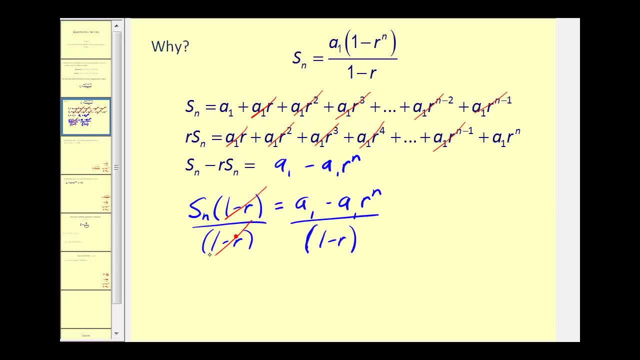 equation by 1 minus r. and now there's only one more step. If we factor out a sub 1 in the numerator, we would have a sub 1 times the quantity 1 minus r to the power of n. I'll divide it by 1 minus r and this is the formula we'll use to find the 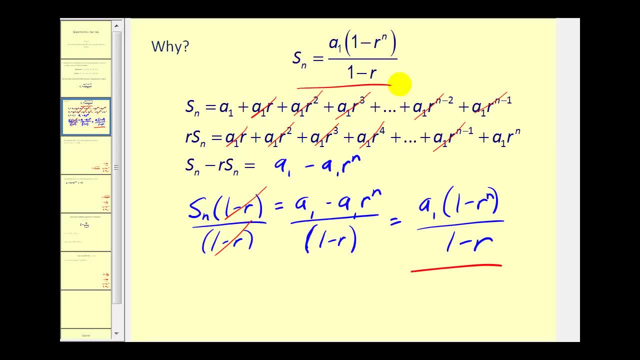 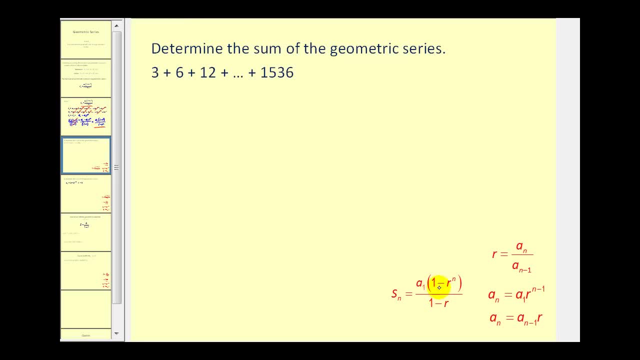 partial sum of a geometric series. Let's go and take a look at a couple examples. Here we have a geometric series. The formula that we're going to use is listed here. We'll have s sub n, or the sum of the first n terms is equal to a sub 1. 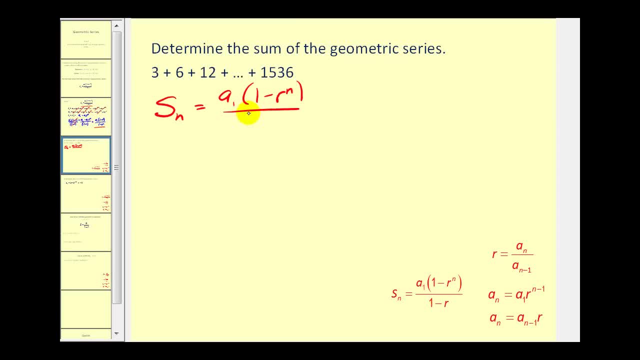 times 1 minus r to the power of n divided by 1 minus r. So we need to find a sub 1, r and n before we can use this formula. Well, a sub 1 is the first term, which is 3.. 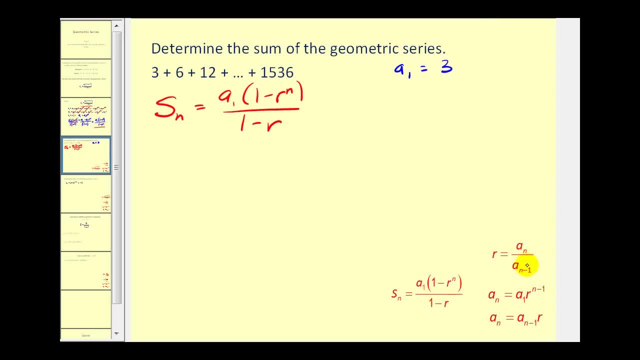 We can determine r by using the formula here, where we select any term in the series and divide by the term before it. So if we use a sub 2, we would divide by a sub 1.. 6 divided by 3 is equal to 2, so r is equal to 2.. 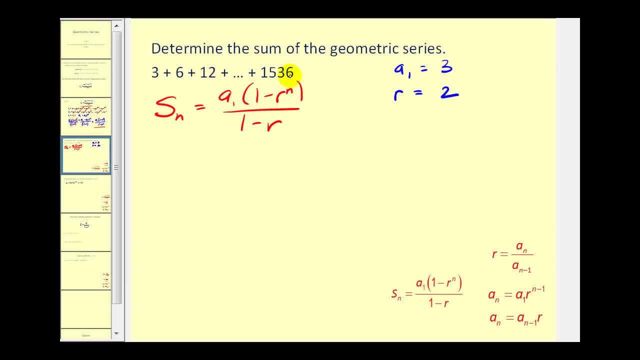 Now we have to determine n, which would be the number of terms in this series. We can use this formula here from our studies of a geometric sequence to determine n. If we let a sub n equal the last term, this n here will represent the number of terms in the 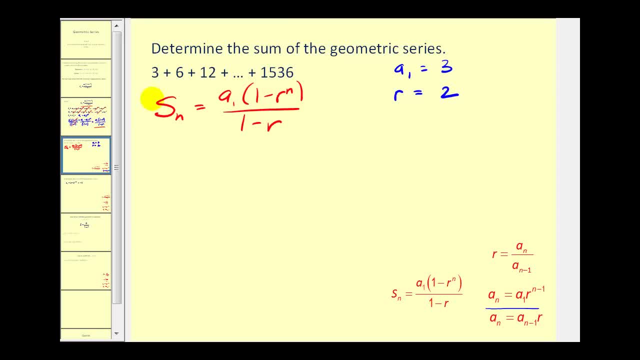 series. So a sub n is equal to a sub 1 times r, to the power of n minus 1.. So a sub n is going to equal 1536.. a sub 1 is equal to 3.. r is equal to 2. And we have. 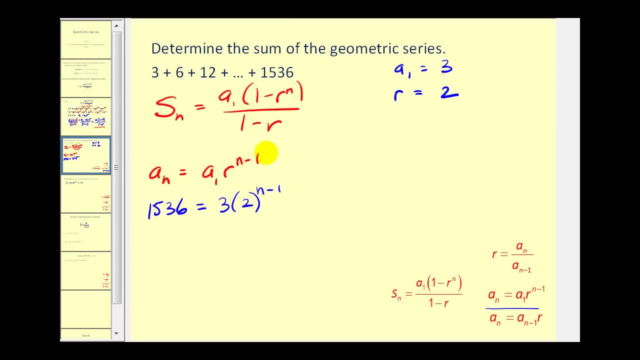 to the power of n minus 1.. We need to solve this equation for n, so let's divide both sides by 3.. This will give us 512 on the left and 2 to the power of n minus 1 on the right. 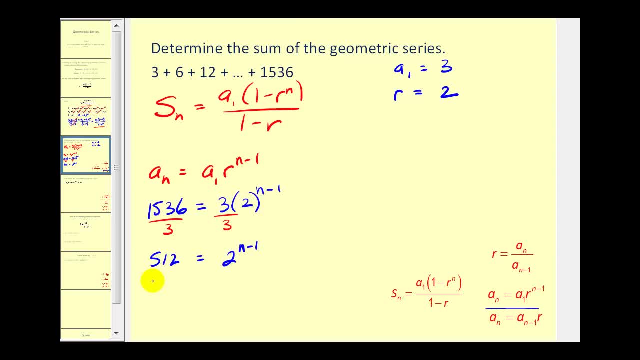 Now, 512 can be written as a power of 2, but we're going to have to divide both sides by 2. It's actually 2 raised to the power of 9.. So from that we can draw the conclusion that 9 must equal n minus 1.. So if we add 1 to both sides of the equation, we know that. 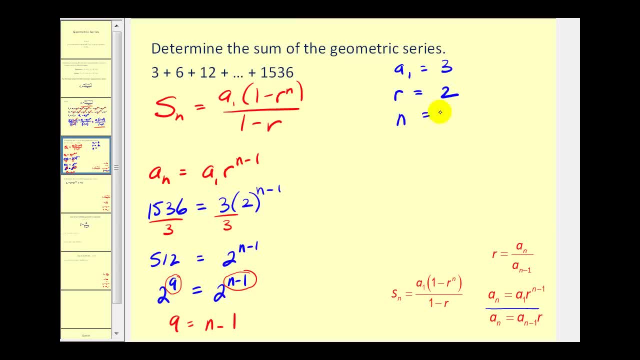 n must equal 10.. This is all the information we need to use this partial sum formula, so let's go ahead and see if we can answer the question now. The sum of the first 10 terms will be equal to 3 times 1 minus r to the power of n or. 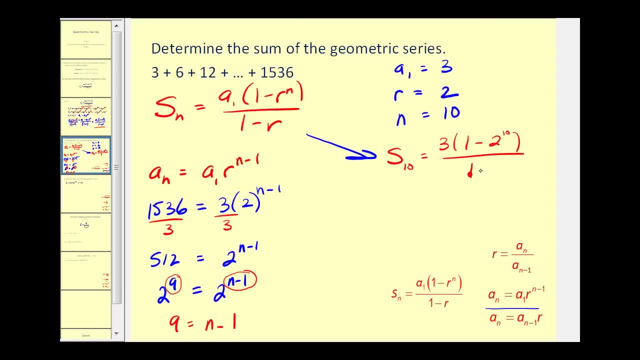 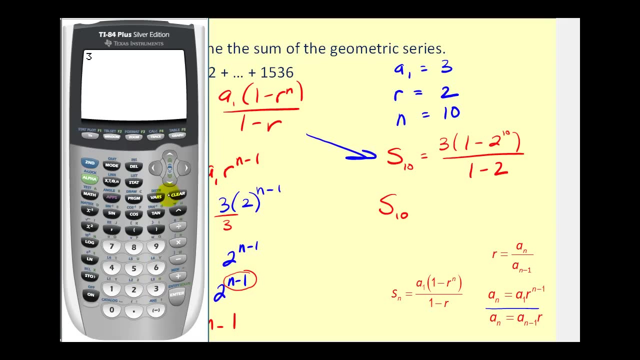 2 to the tenth divided by 1 minus r, which is again equal to 2.. Let's go ahead and go to our calculator and see if we can determine this partial sum. Let's take a look at the numerator first. We're going to have 3 times the quantity, 1 minus 2 to the power. 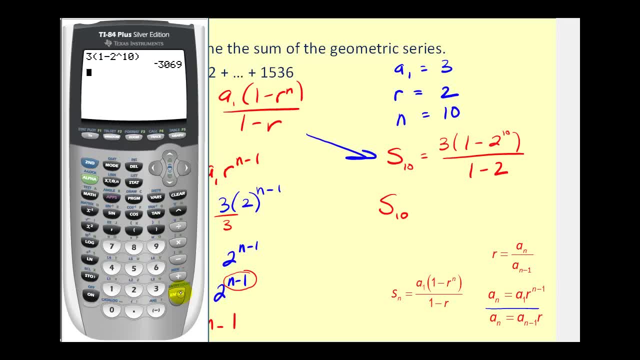 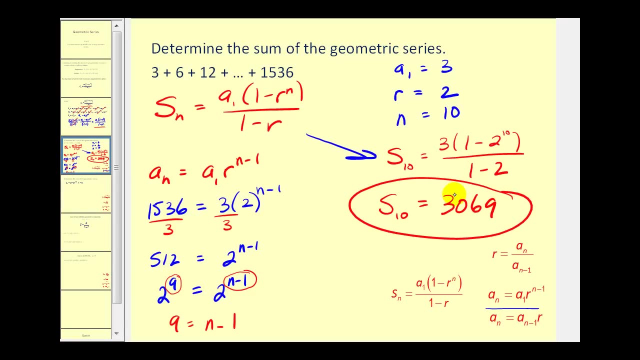 of n of 10.. There's our numerator, And we're going to divide by 1 minus 2, which of course is negative 1.. So we have 3,069 for this partial sum. Let's go and take a look at another example. 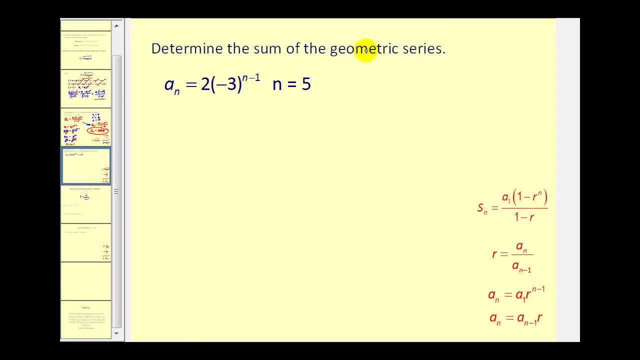 On this problem. we have the formula that will generate the terms in the series and we also know there will be 5 terms, because n is equal to 5.. So again, let's write out our formula. We want the sum of the first 5 terms, because we know n is 5.. So to find 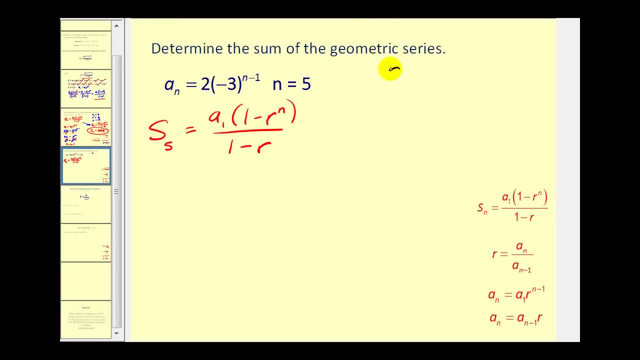 the first term we're going to have to use this formula: a sub 1 is equal to 2 times negative 3 raised to the power of n minus 1.. Well, if n is 1, 1 minus 1 would be 0.. 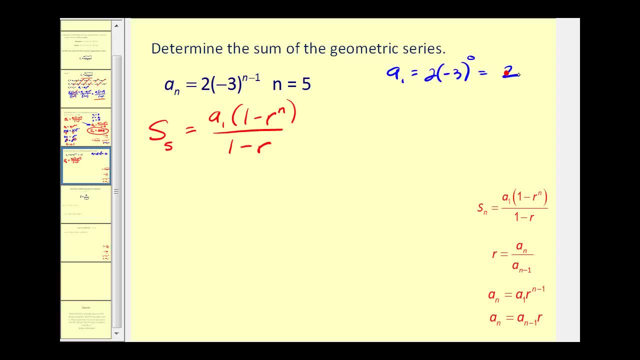 Negative 3 to the 0, power is 1, so we have 2 times 1, or 2.. Now we do have to find r. If we can't look at this formula here and see what r would be, we would have to find one more term so we could use this formula here to determine. 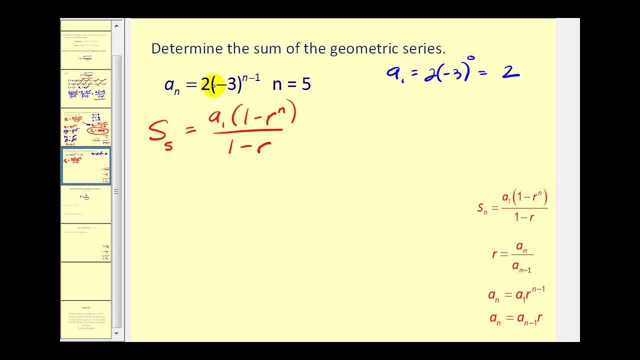 r. Let's assume we can't determine r by looking at the formula. Let's go ahead and find the second term. So we have 2 times negative 3 to the power of 2 minus 1, or to the first power. Negative 3 to the first is negative 3 times 2.. That's negative 6..